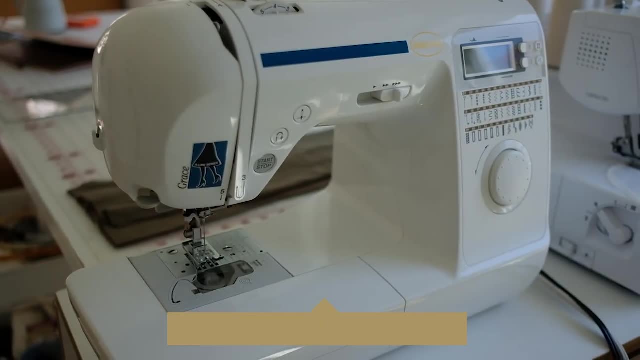 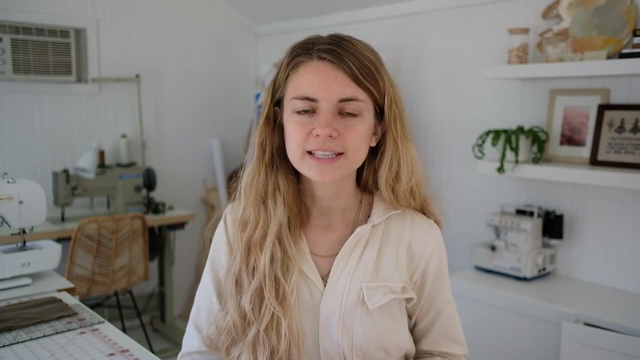 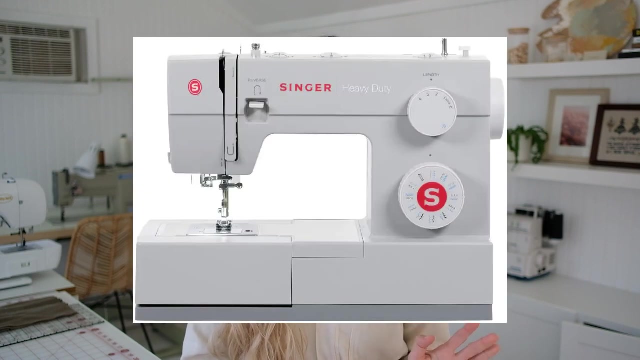 So I'm personally using a Baby Lock Grace and for you I would recommend starting with Baby Lock Joy. The Baby Lock Joy will have all that you need to get started and it is at a great price point, under $200.. The Singer 4423 is just a classic heavy duty sewing machine and this is a great way to get. 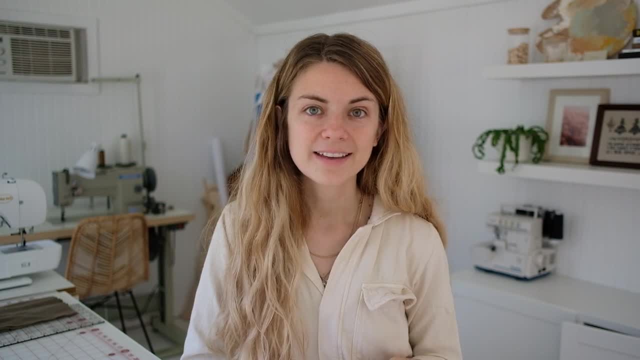 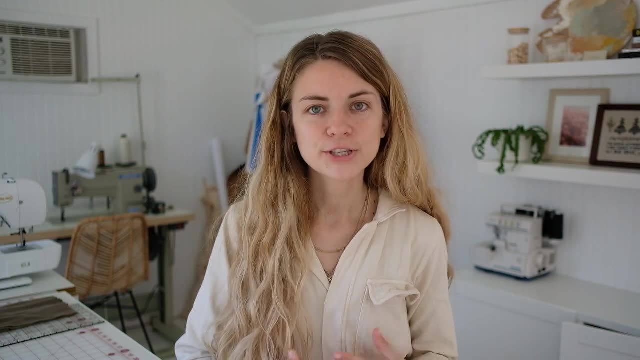 started. It's under $200.. I highly recommend it if you just want a very basic machine that will stand the test of time. Another trusted machine is the Janome 2212.. It comes with a lot of extras within it and it's also. 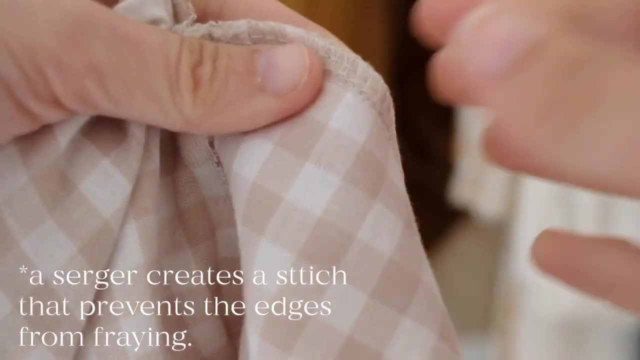 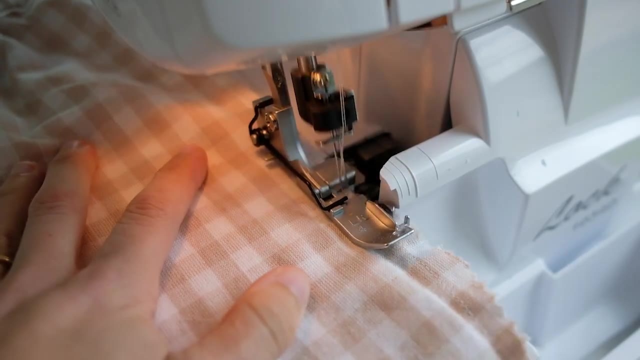 under $200.. Just note, you don't need a serger to get started, but if you're looking for one, I recommend the Brother Serger, and I have it myself. I love it. It makes things so much easier. It's so great. if you're making a lot of clothing that you'll be washing and wearing on a Sunday, You'll have a lot of. 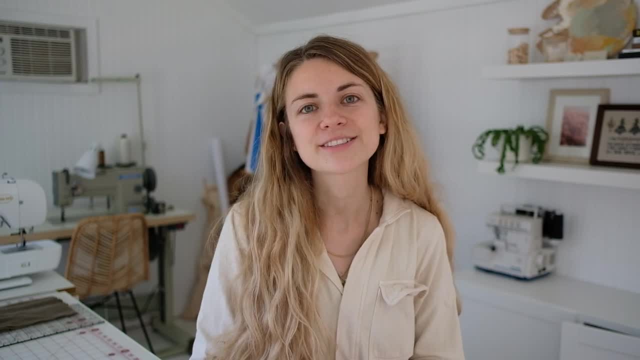 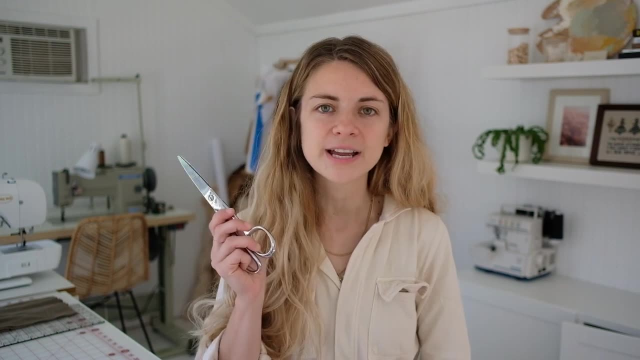 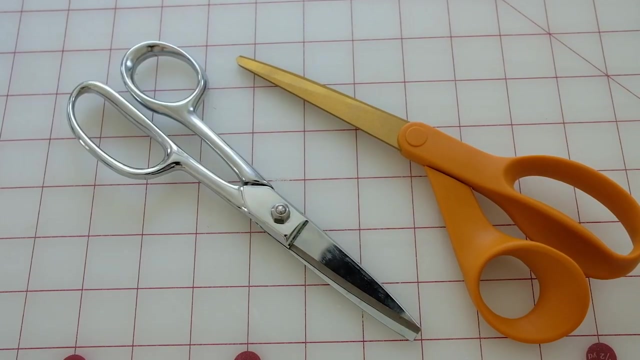 and wearing often. but just know, you don't need a serger to get started. it's just a recommendation for the future. the next tool that you'll need is scissors. so you want a good pair of scissors, and these will only be used for fabric. you want fabric scissors and you can write on them. 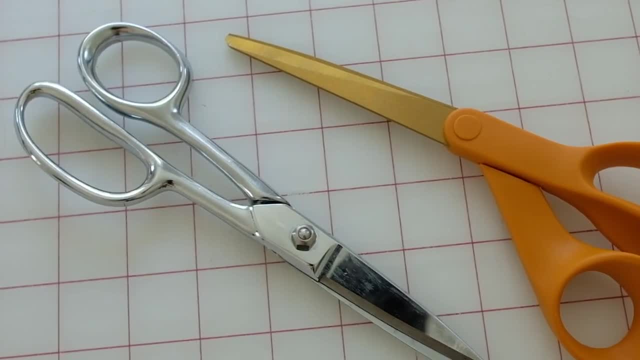 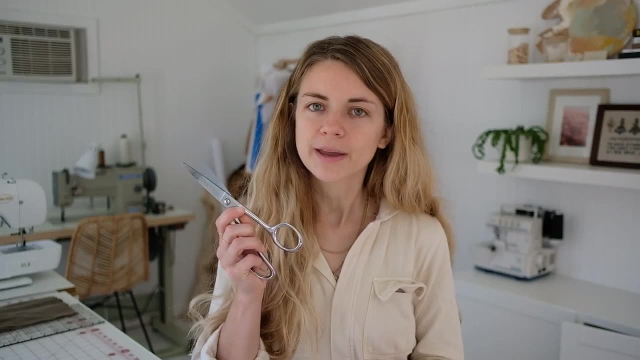 tie a piece of string around them. just make sure that you and everyone that is going to come in contact with these scissors know that they're only for fabric. so i actually have a pair that are supposed to be for fabric only, but through the years they kind of got picked up. 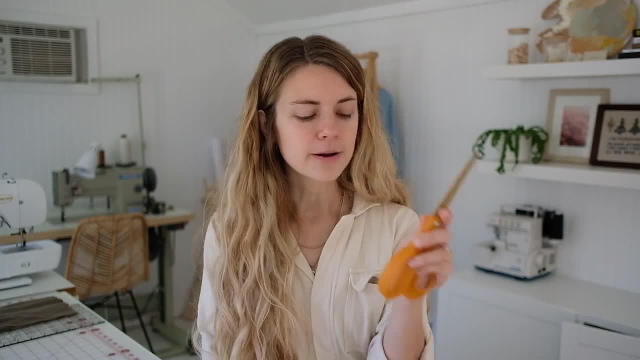 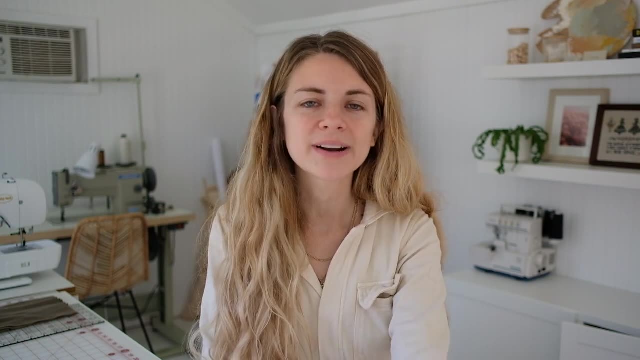 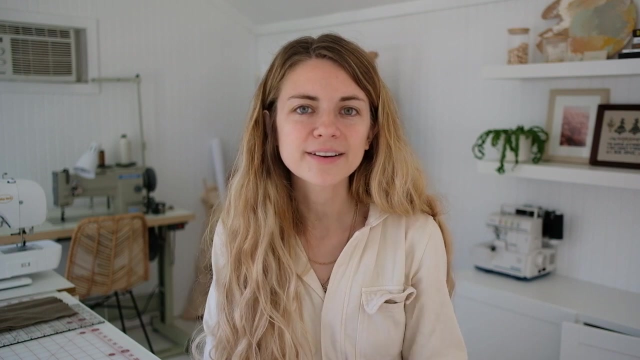 and i don't use them for fabric anymore. so i have my own fabric scissors and i i protect them. so when you have fabric scissors, you don't want to use them on paper or anything else, especially plastic, because it's going to dull the blade. a good pair of fabric scissors will last you years. 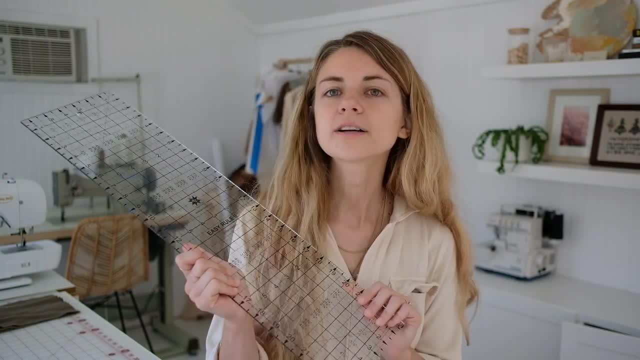 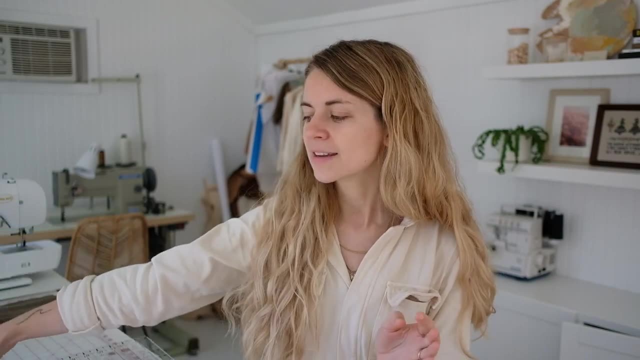 and you can also get them sharpened if you need moving right along to a straight edge. i love the clear straight edge, but for a while i use just a right angle and that is all you need to cut out straight lines. i love this clear one because 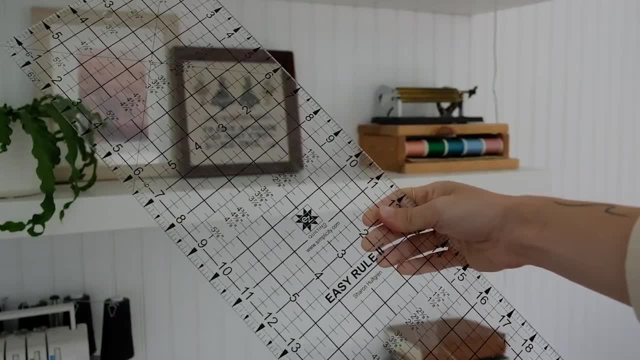 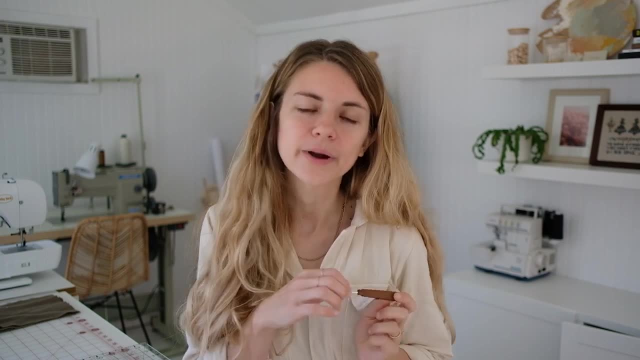 it helps measuring things a little bit better, and i think it's under the quilting section. so keep an eye out for that when you're at the fabric store. you're also going to need a seam ripper. i use this on probably every project because you'll get going. 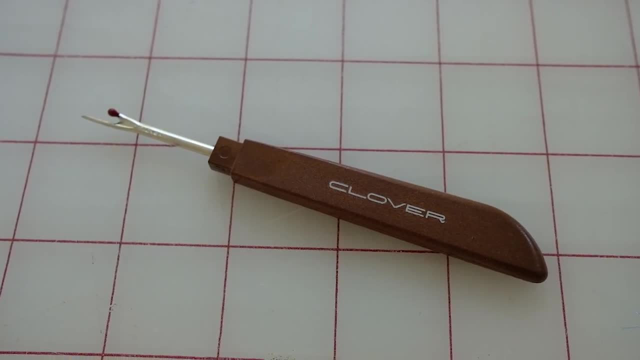 you're not thinking about it, and then you'll sew something you're not supposed to. but it's really easy to use. you'll need a seam ripper- pick one up, they're a couple bucks- and you'll also need a piece of fabric that you can use for sewing, or you can use it on the fabric, but i'm not going to. 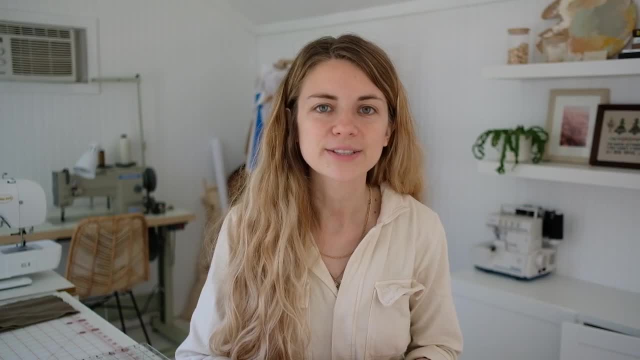 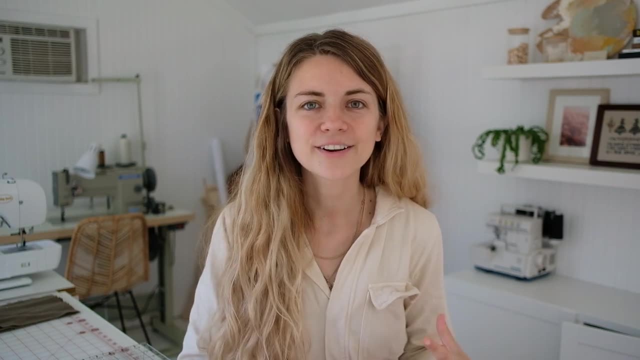 need some pins, especially if you're making something out of a pattern. It's great to cut fabric and pin things together when you're about to sew, so definitely pick up some pins. Ironing your garment along the way as you're sewing is going to yield a much better result, So you can. 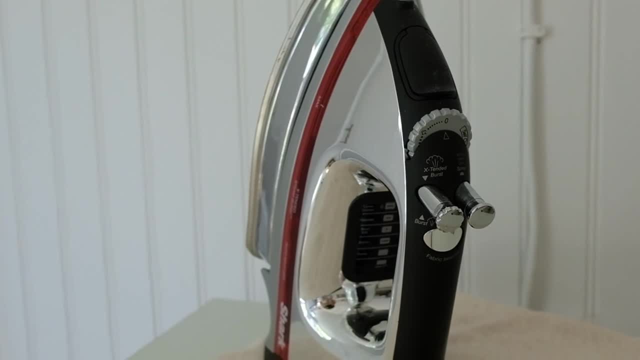 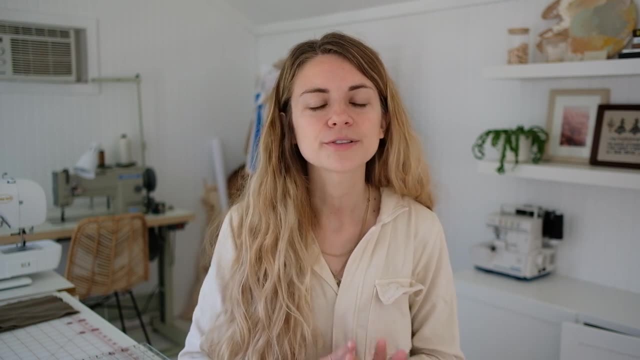 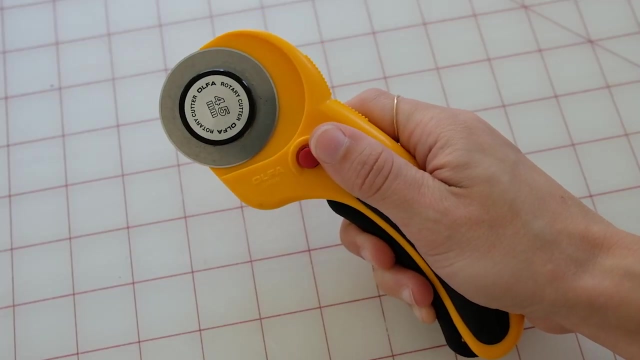 use an iron. I just use my home iron- Nothing fancy. You can get a heavy duty iron if you're interested in that, but a good iron will help your project turn out so much better. You'll also want a measuring tape, and a rotary cutter is also great for cutting long lines, and some people 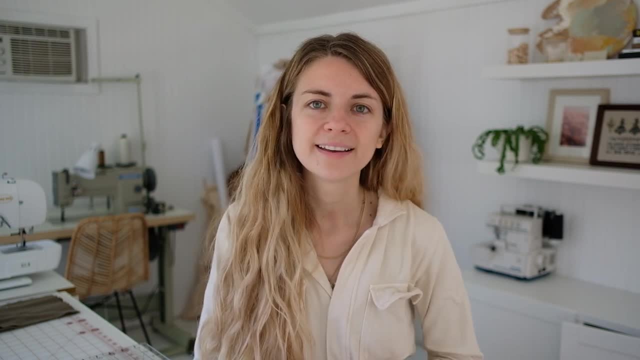 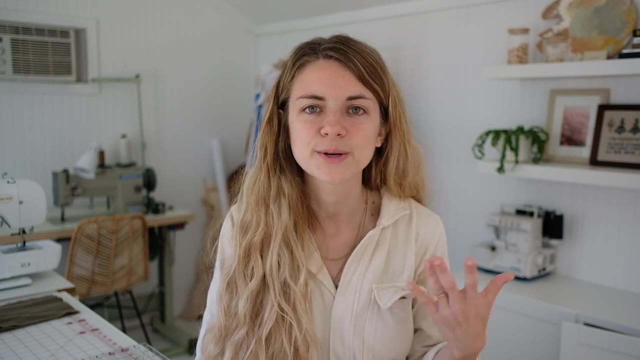 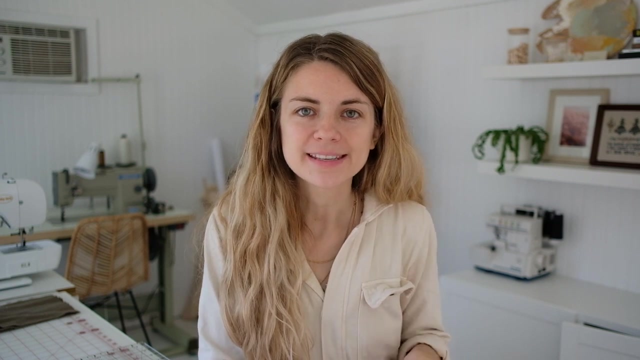 prefer to cut out all of their patterns with a rotary cutter. It's up to you. You can also use scissors, but I definitely recommend the rotary cutter for cutting out straight lines with your straight edge that I mentioned earlier. Now let's move on to the basics of getting started To thread. 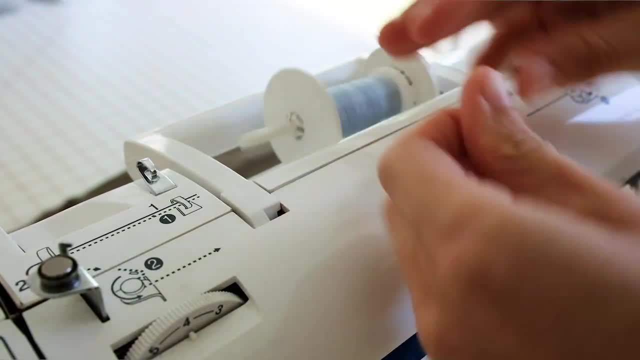 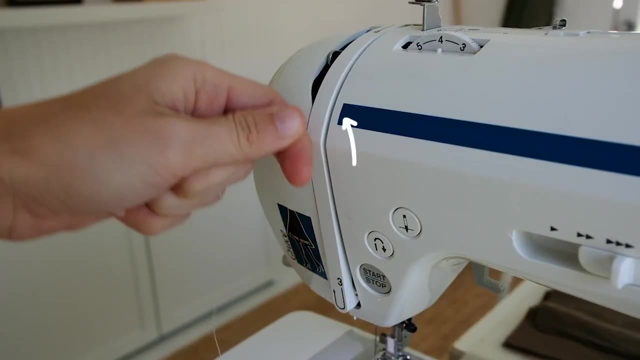 your machine. you're going to start with your thread, You're going to start with your spool and then you're going to guide it throughout the whole machine, following the numbers that are indicated on your machine, and go all the way to the needle. 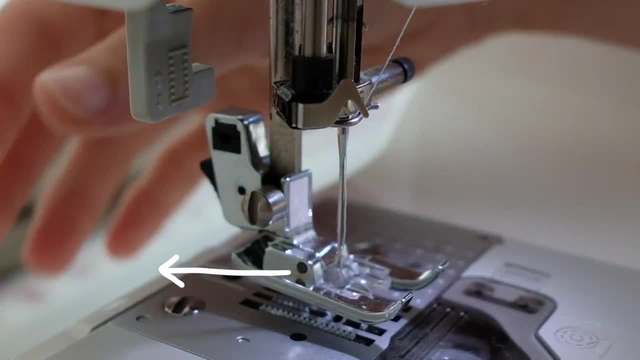 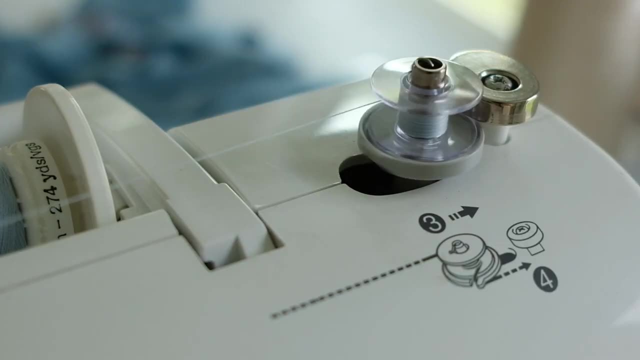 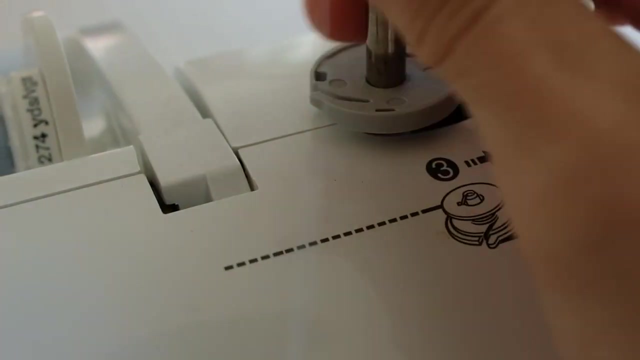 Every machine is different, but the basic principles are the same. Don't forget to add the bobbin and make sure it's the same color as your thread, So you can wind the bobbin beforehand and you do the same thing you would to thread the machine and you just follow the numbers and allow the machine to. 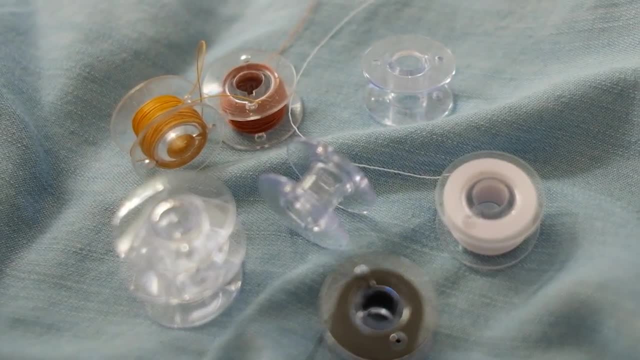 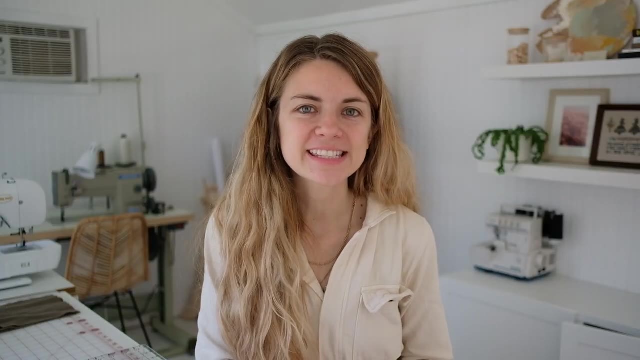 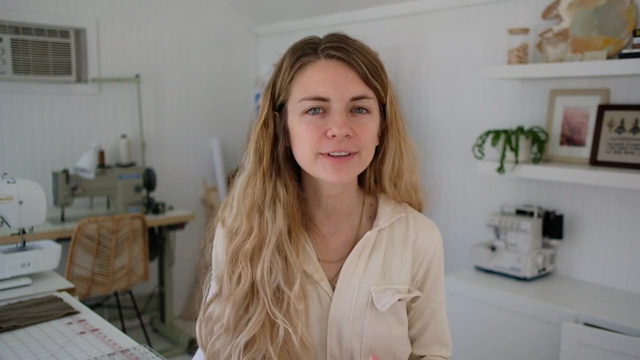 go. I recommend having different bobbins on hand when you're switching out colors, so it makes things a little easier and you can save colors and not waste that thread. A straight stitch is the very basic stitch that you're going to need when sewing anything You'll definitely change up. 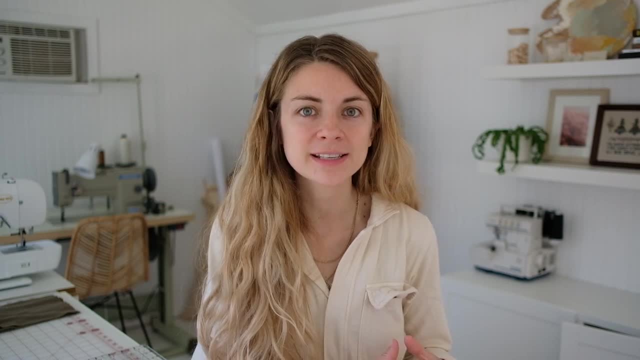 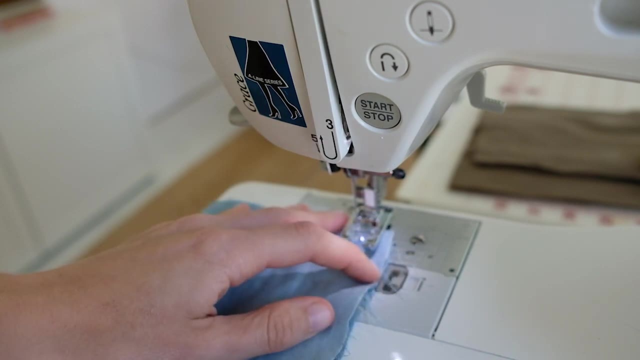 the stitch, depending on what project you're doing, but the straight stitch will take you very far. So, to start out, you're going to slide your fabric under the presser foot and lower the presser foot. You're wanting to make sure, with whatever pattern or project you're following. 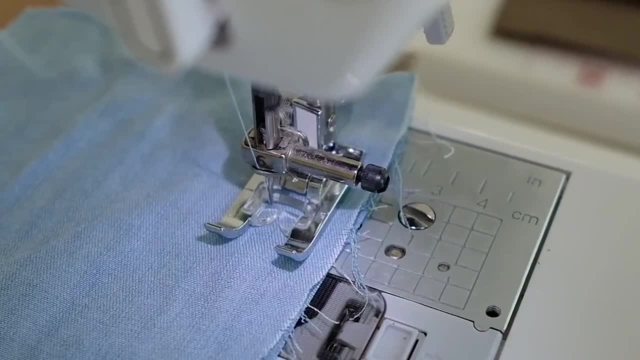 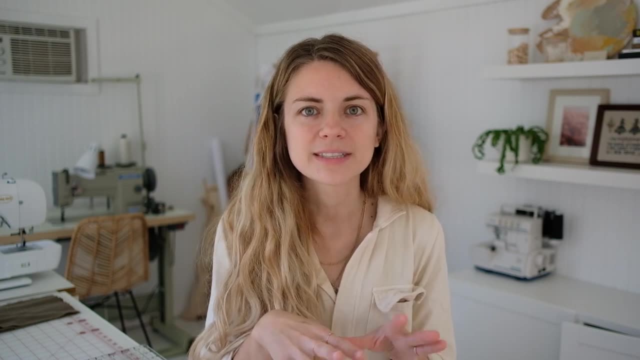 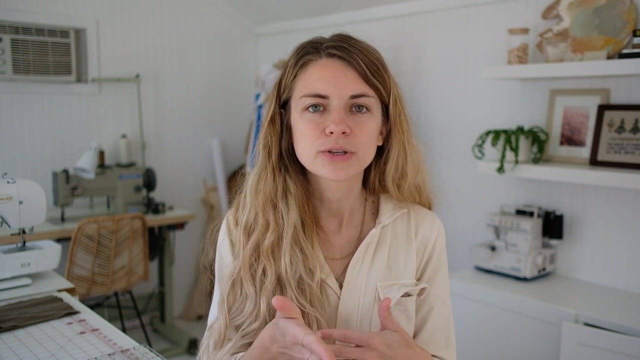 if it mentions the seam allowance. you want to follow this. So you're going to line up your fabric and the presser foot and the needle where the seam allowance shows. So if it's half an inch seam allowance or a quarter of an inch or 5, 8ths, you want to line it up and usually on your machine. 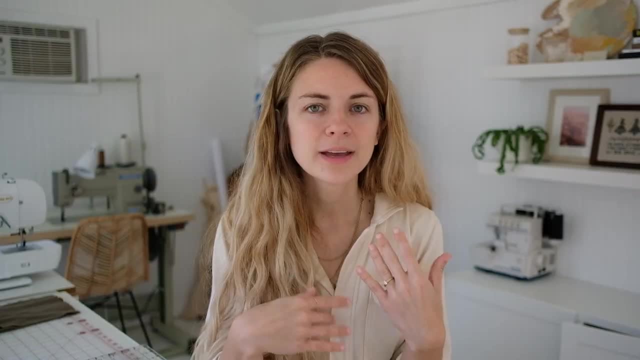 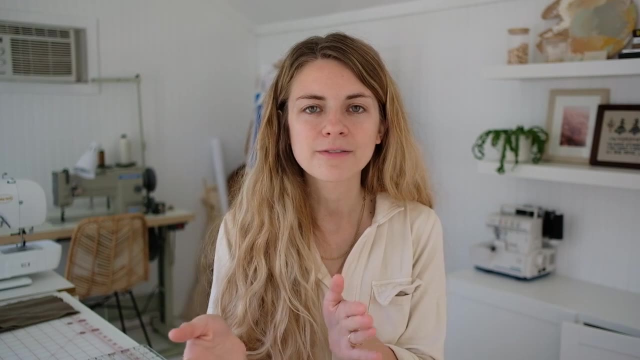 there is a little ruler or measuring tape to show you, And if not, you can just take out your measuring tape that you have. And then you're going to take out the measuring tape and you're going to measure where the needle is to the end of the fabric. To start out, you always want to do a. 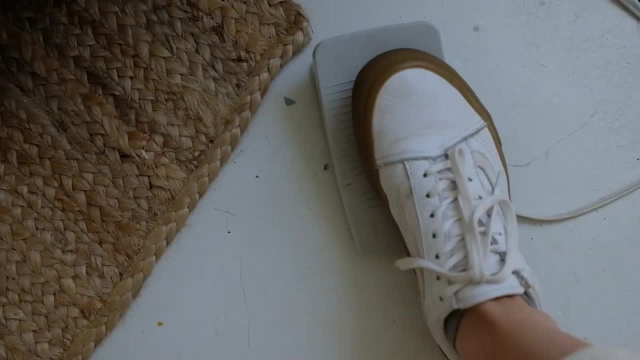 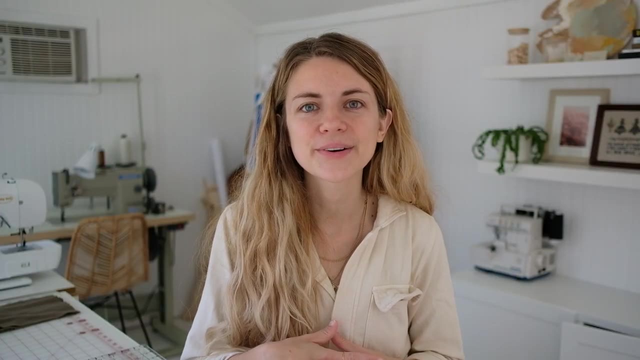 back stitch. So you're going to start by pressing the pedal with your foot and going slow. So, gently, press it like you're pressing the gas pedal in your car and you're going to start stitching. It's going to go very slow at first. All you want to do is make two to three stitches. 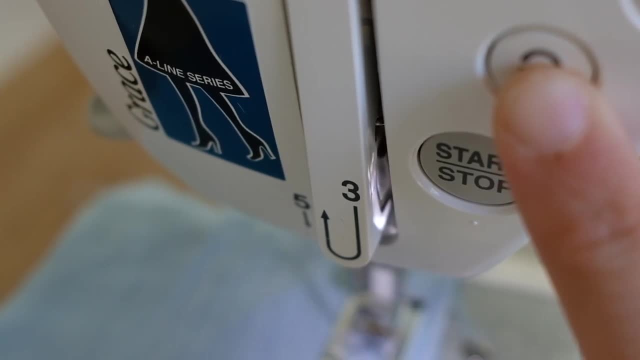 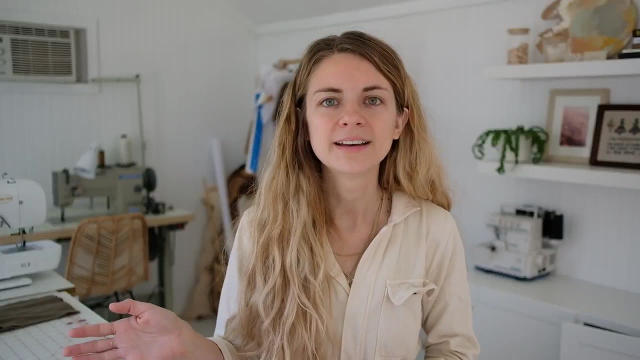 and then you're going to stop, press the reverse button on your machine and go back two to three stitches. This is going to give you the same length, and then you're going to go forward and keep sewing. You're going to do this when you reach the end of your project and you're going to reverse stitch. 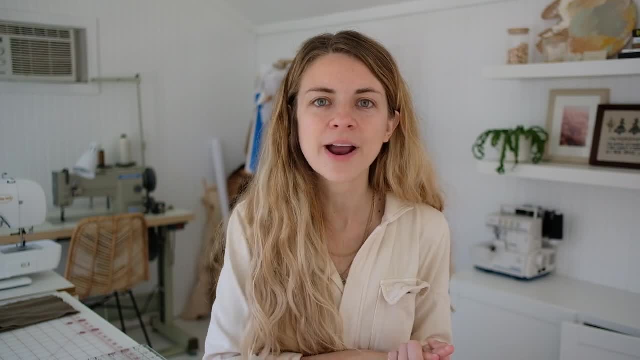 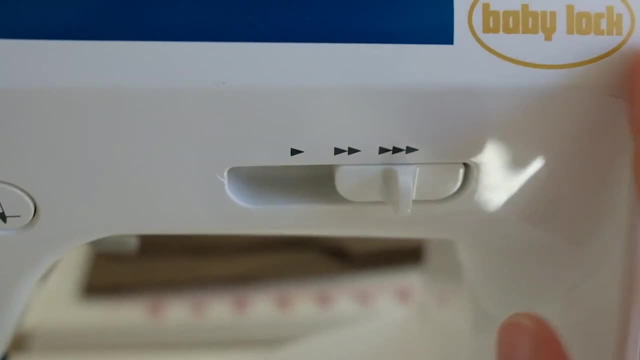 once more, And this is going to lock your stitch in place so it doesn't unravel or come undone When you're starting out doing your straight stitch. you want to go really slow. If your machine has like a speed regulator on it, I recommend going to the very bottom speed. 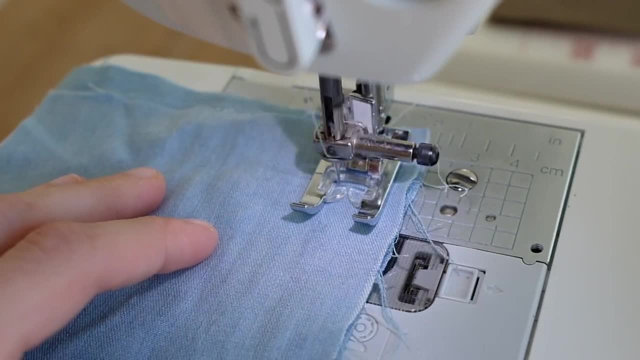 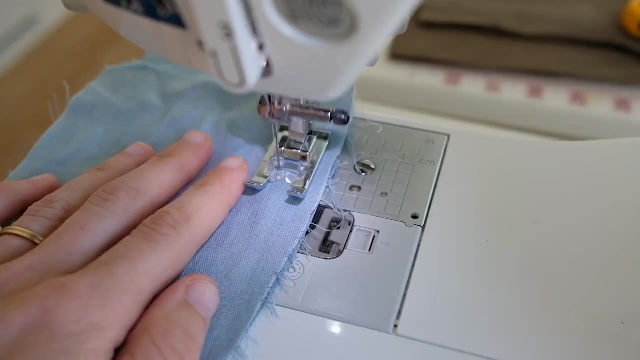 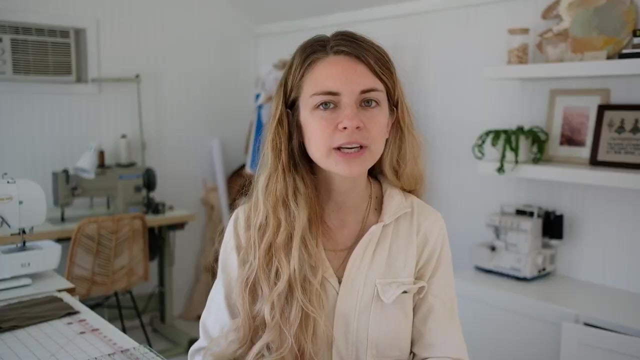 and going just one stitch at a time, lining up the stitch with the seam allowance originally started with. so doing this is just gently guiding the fabric through the presser foot at slow pace, not gripping the fabric, not pushing it through, just allowing the machine to guide it through. the machine will do the 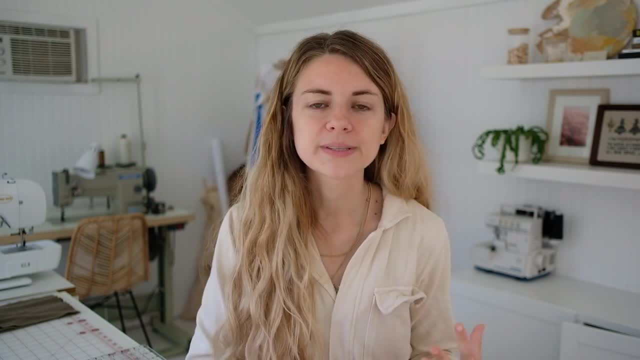 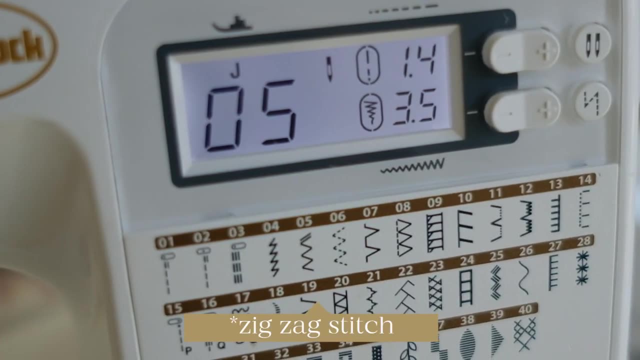 work and all you have to do is guide it. so these same principles work for the zigzag stitch as well. this is a stitch that I recommend you looking for when you're buying a machine, because it will come in handy and a lot of projects. so when you're doing a zigzag stitch, you'll still do the reverse stitch. 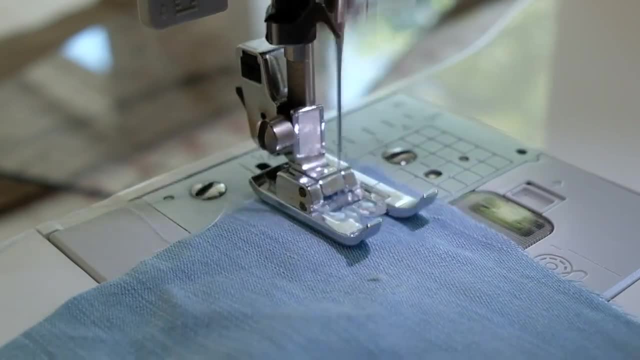 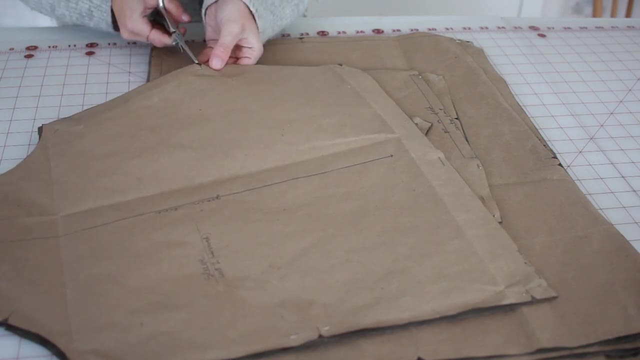 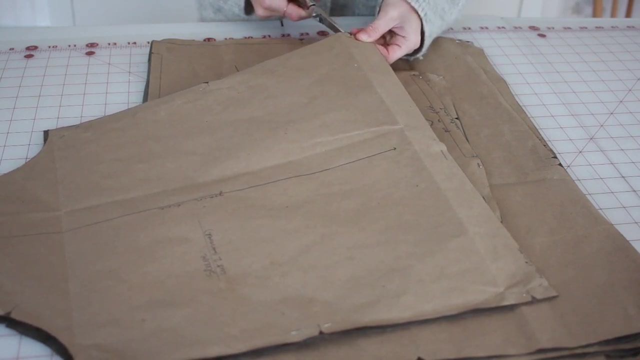 you'll go slow, you'll guide the fabric and let the machine do its work. another technique that a pattern might call for or a project might call for is just making notches. so this is just taking your scissors and making a little snip at the edge of your fabric, and this is either to line up the pattern or it's to. 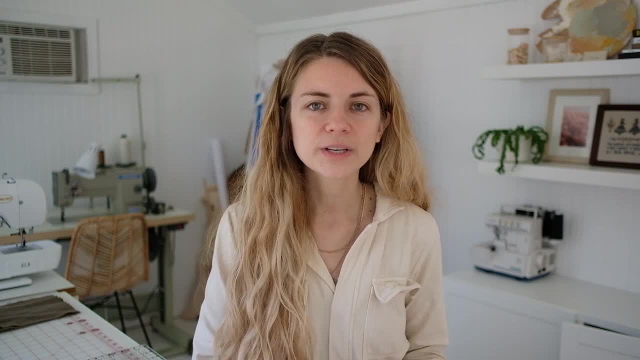 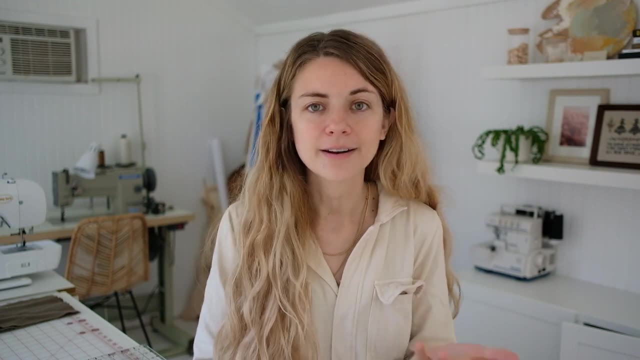 make it the curve lie flatter, and you want to make sure that the curve is not too high or too short. so if you want to do this, your project will usually show you where you need to do this. we all mess up a seam here and there or on. 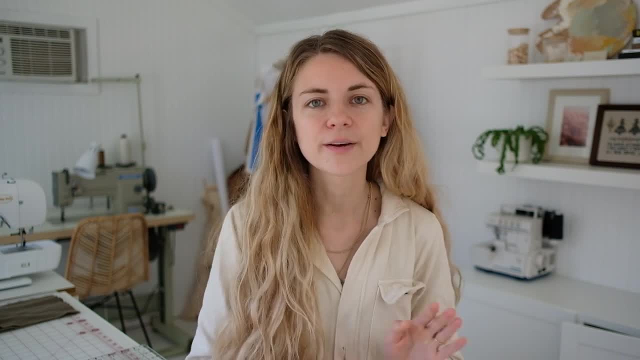 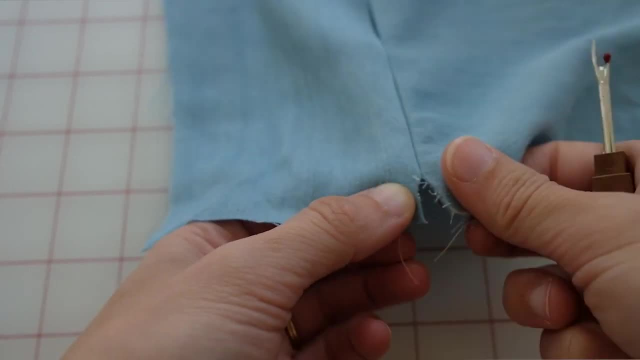 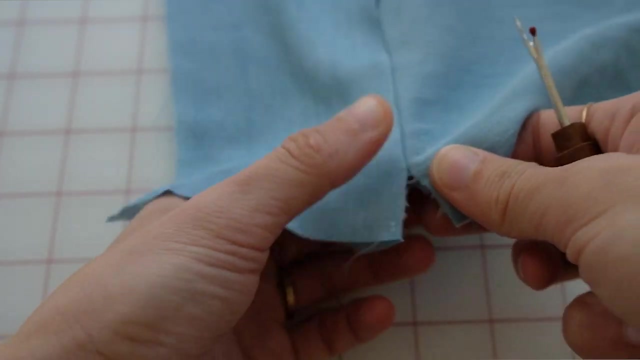 every project and so you'll want to seam ripper, like I mentioned earlier. so you just take your seam ripper and flatten out the seam. so you want to carefully insert the tip into your seam- and that one has already been sewn- and just carefully guide it through and a little bit of pressure and that's going to rip. 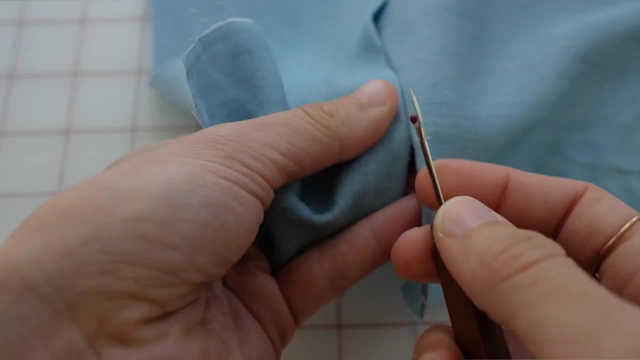 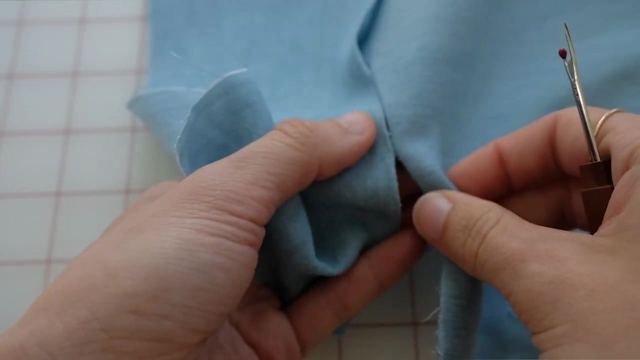 those seams apart. This little red side is on the bottom and this is going to make sure you're not puncturing the fabric in the wrong place and creating a hole. Make sure you're going slow and then at the end you can pull out all the extra threads. 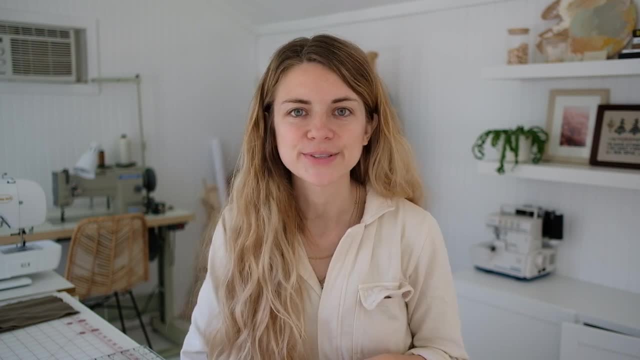 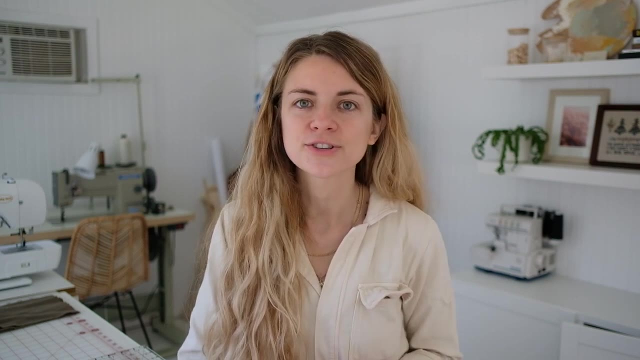 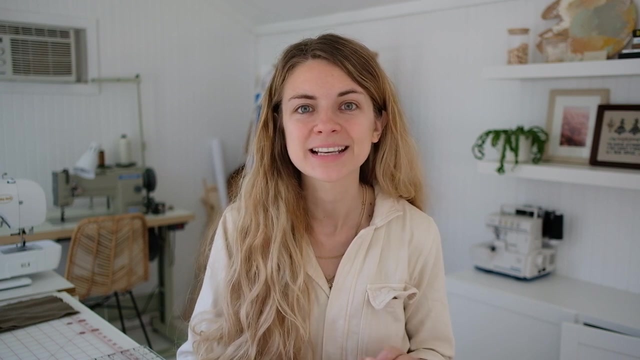 Now I want to suggest a few projects to get you started. With any project, it's really about starting and going through the detailed instructions and reading over them before you get started And starting with a project that you're going to be excited about, excited to pick back up, excited to finish. 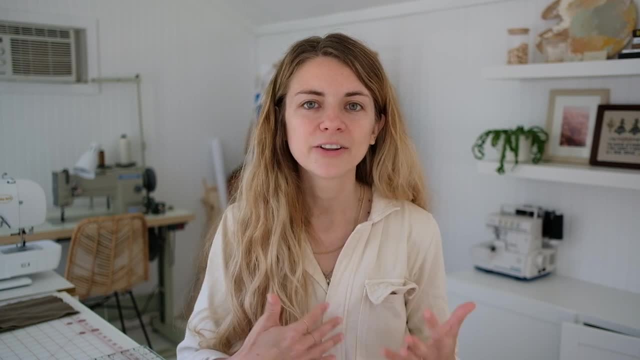 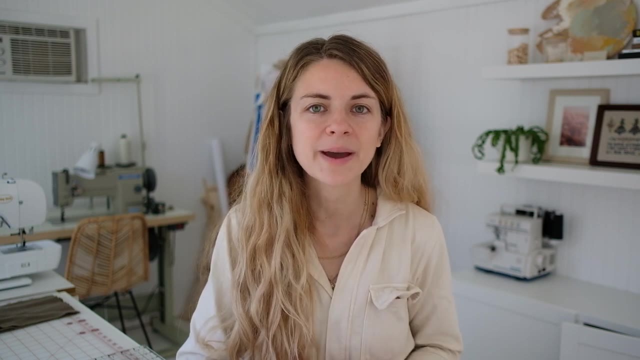 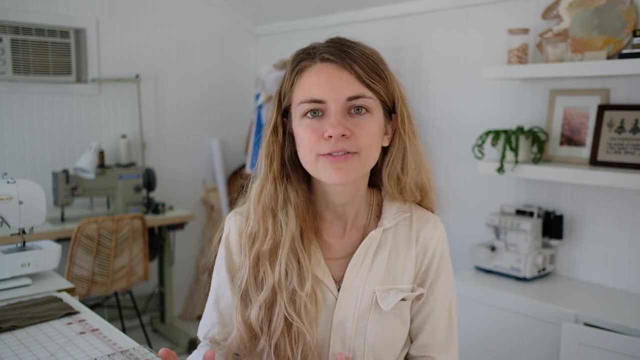 And so that's why I'm going to recommend a lot that I've already made here on videos, because they have detailed instructions for you. Some come with patterns, and in them you're going to learn some basic skills that are going to carry over to every project that you make from now on. 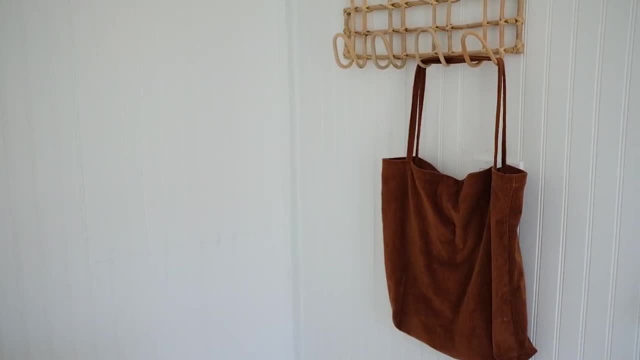 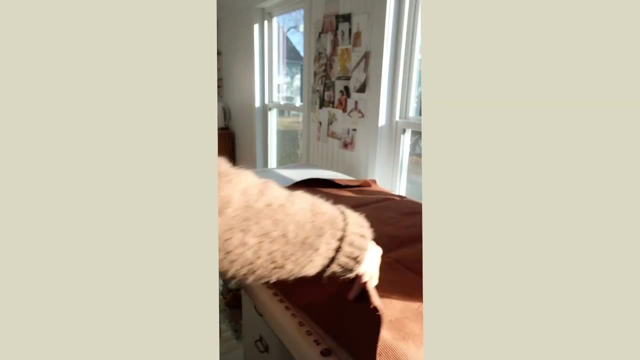 First project is a tote bag. I'm going to insert the video now on how to make this tote bag. Here is how to make a super simple oversized tote bag. You'll need one yard of fabric and you're going to cut that to measure 21 inches by 36 inches. 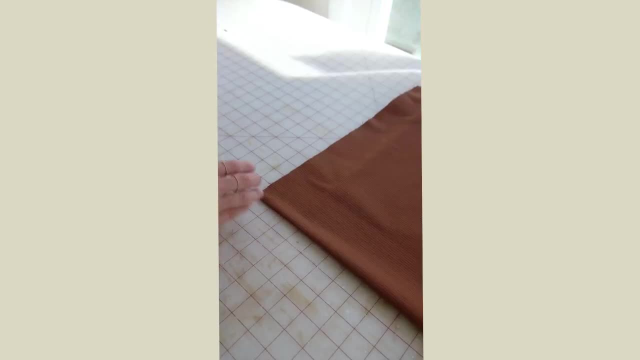 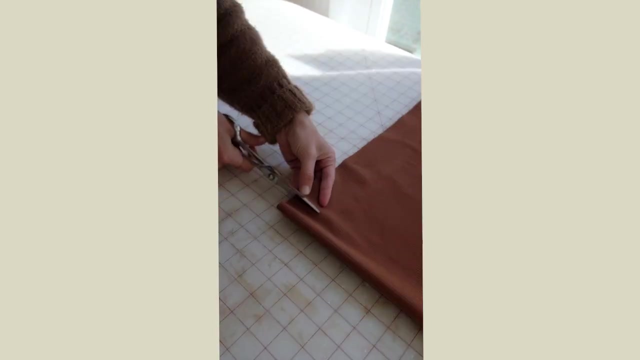 Fold this rectangle in half and from the bottom of the fold you're going to measure one and a half inches up and then one and a half inches over, You're going to cut the slit and then sew along the sides, from the top of the tote down to the cut you just made. 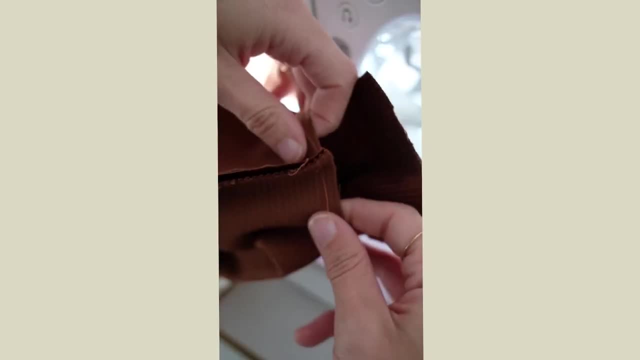 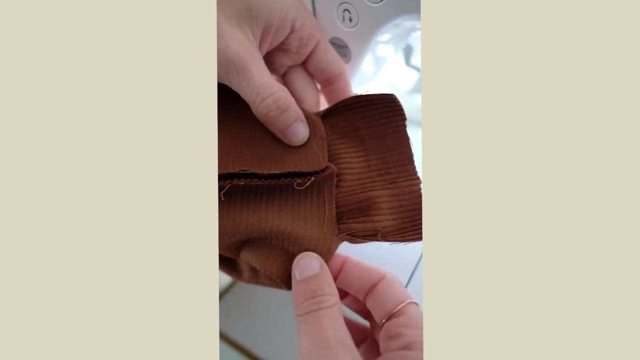 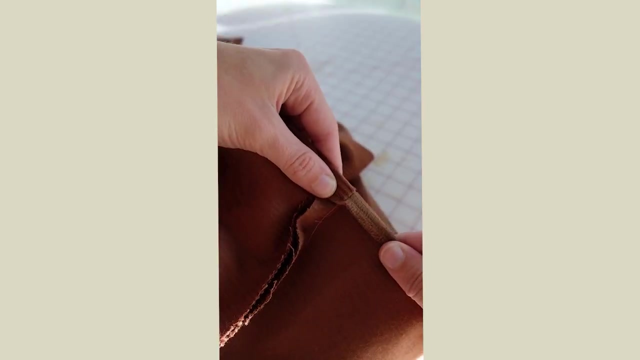 Repeat this on both sides, and then you're going to open up the tote, where you are flattening out the seam on the bottom, and then you're going to make this a little flatter and sew along the sides. Now, from the top of the bag, you're going to fold over once, about a quarter of an inch, and 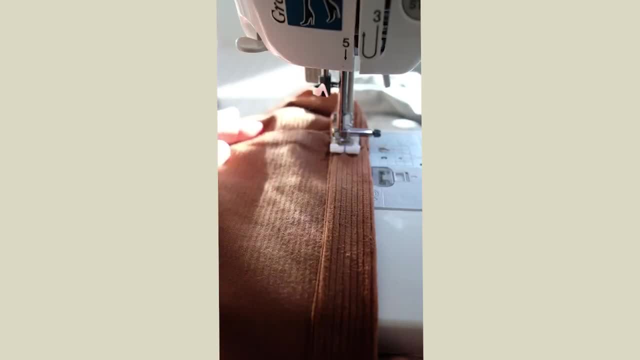 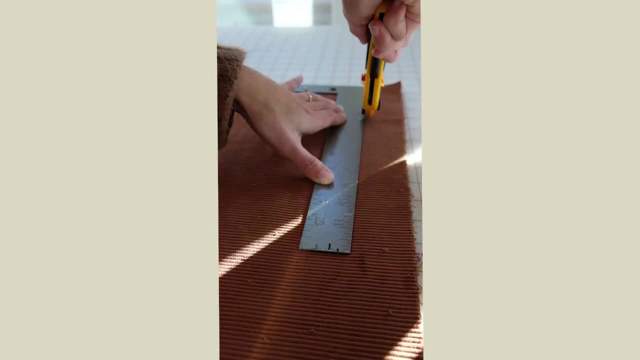 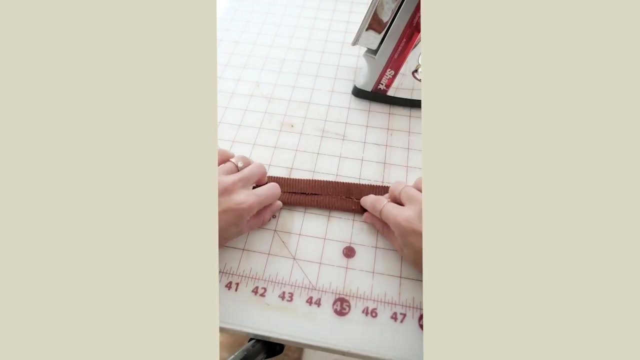 then fold it again another quarter of an inch. Then you're going to sew along the entire edge of the top of the tote To make the straps. you're going to cut two strips that measure 22 inches by 3 inches, Fold these straps in thirds and then fold them once more onto itself. 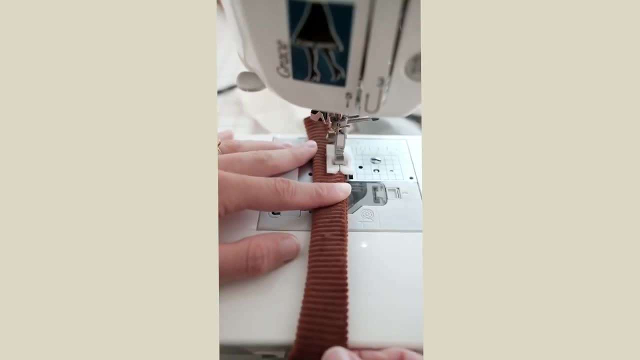 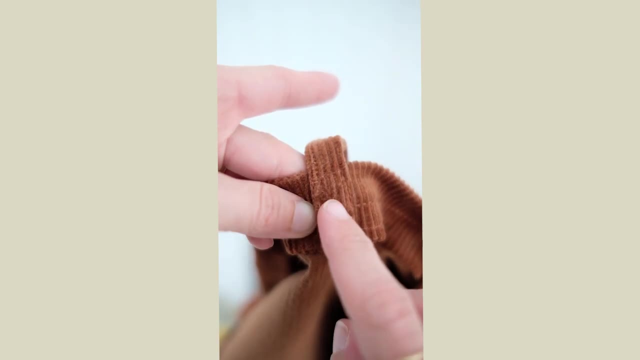 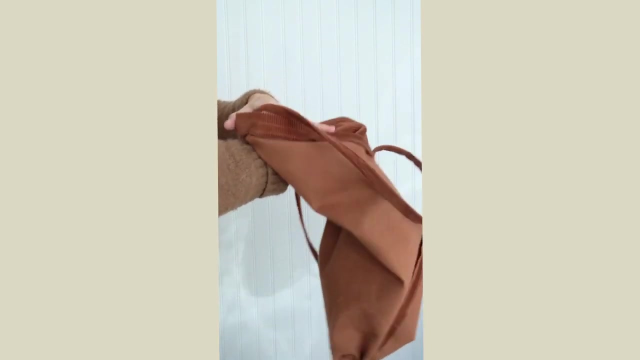 Sew along the side and you'll have two long straps. Then you'll attach this to the top of your tote bag and make sure you're just securing it by sewing it in an X and rectangle formation. Finally, you will turn your bag right side out and you're all finished. 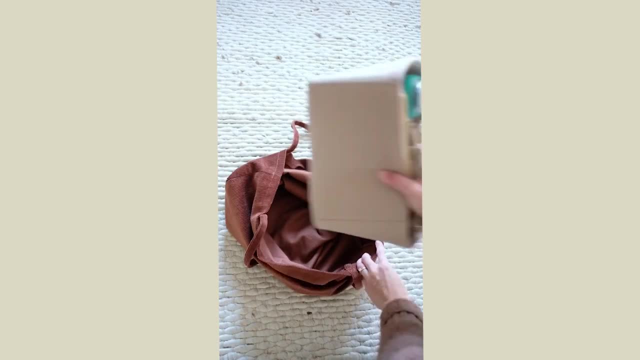 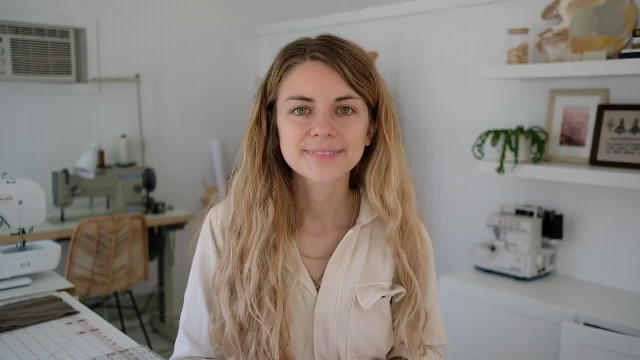 I like to add a organizer to my bag so I can find things a little bit easier and move my organizer from different bags that I use at different times. If you're making a project for a little baby or a little child, I suggest the Rhodes overalls. 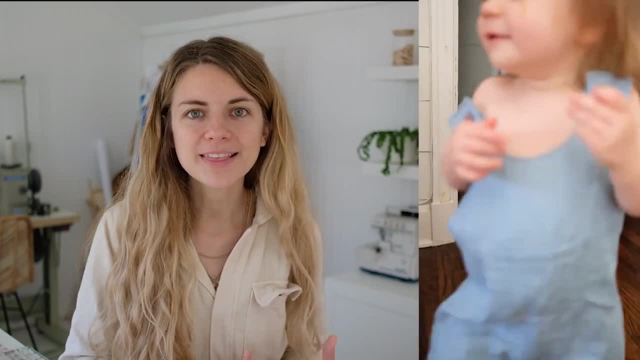 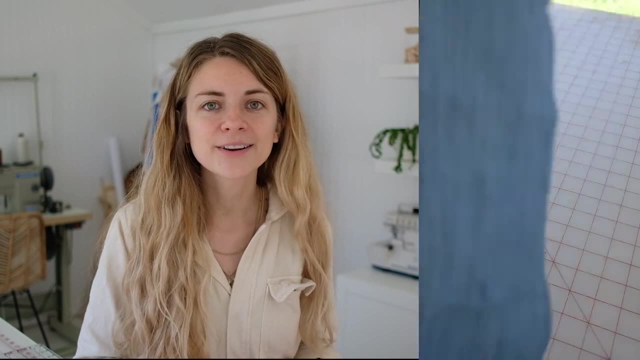 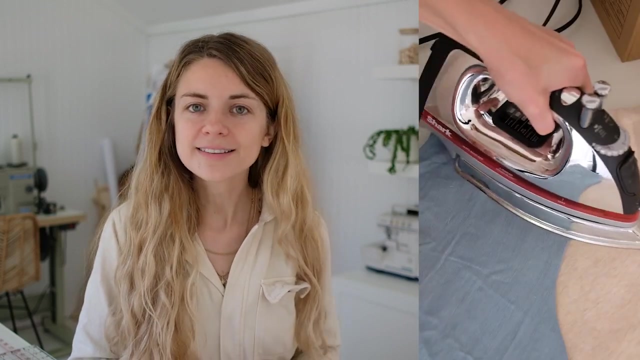 These are so simple to make and once you make them, you'll learn not only how to put a simple piece of clothing together that your child can wear. you'll learn elastic casing and how to add elastic to any garment. You'll learn how to add a button which is not as scary as it sounds. 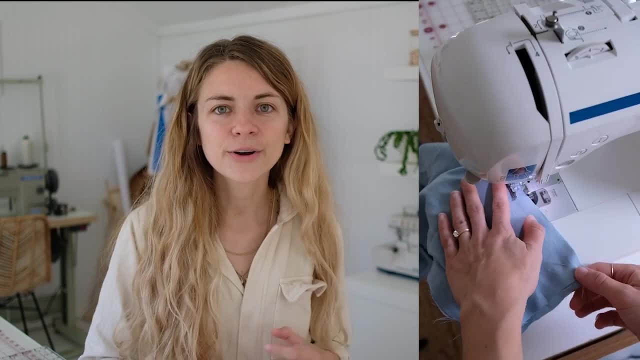 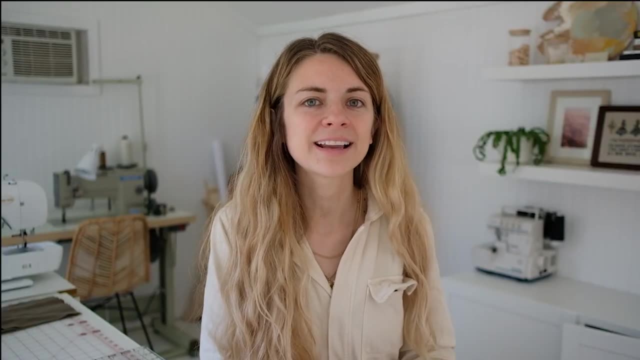 You'll learn how to do a pocket and all of these things are included with the pattern. There's a video for it on our channel and you can also find the pattern at runyclothingcom. A birthday crown is also super simple to make. 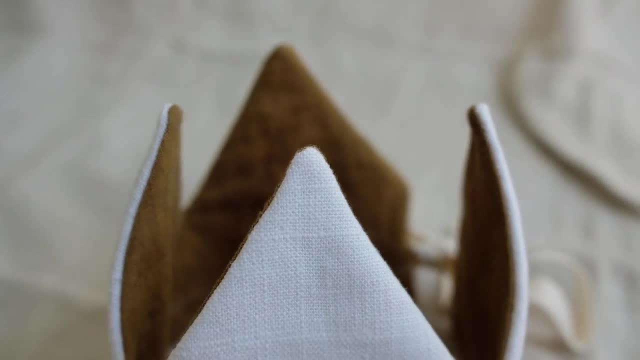 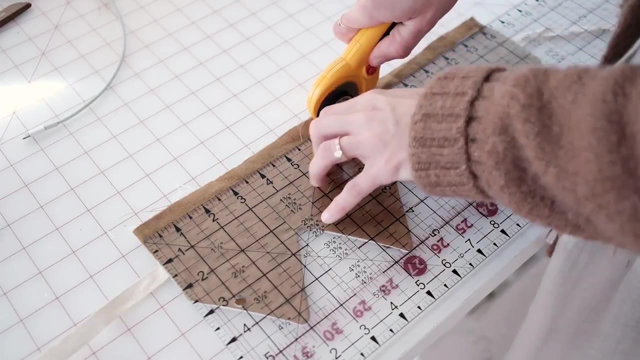 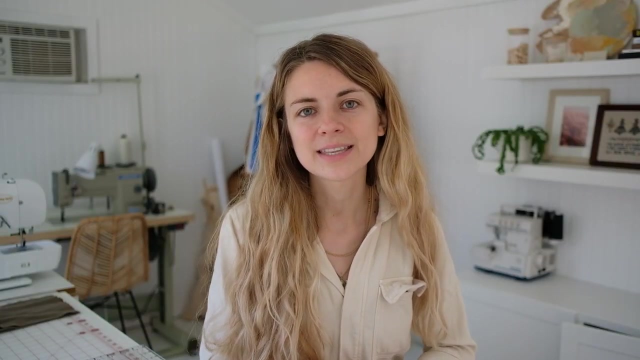 This is going to take you less than an hour. if you're a beginner, It might only take you 20 minutes. This is a great project: learning how to do it, How to sew points and making sure they're pointed. This will also show you how to add binding and add a little ribbon detail to the back.